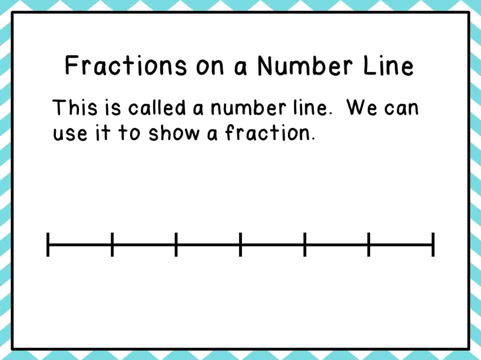 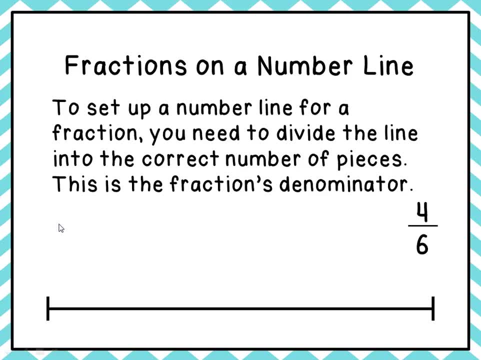 number line. we can use it to show fractions and sometimes this: this is just a line and we've broken it up into two pieces. Now, to set up a number line for a fraction, you need to divide the line into the correct number of pieces, And we find this out by looking at the fraction's denominator. 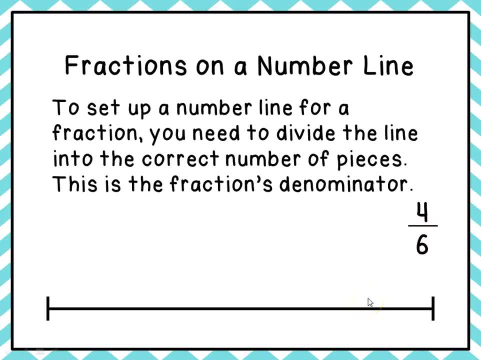 So over here you can see that the denominator is six. so what we need to do is we need to divide this line into six different pieces. There's two pieces, three pieces, four pieces, five pieces and six pieces: One right here, two, three, four, five and six. It's very. 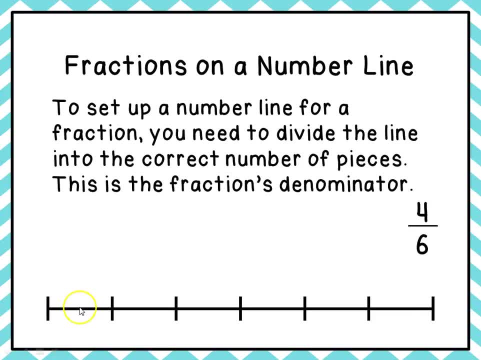 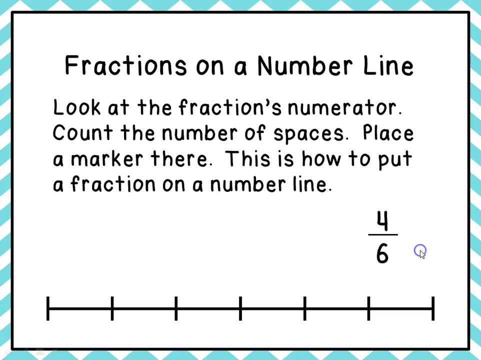 very important that you always count the pieces and not the lines. here You don't count the lines, you count the pieces. So one piece, two pieces, three pieces, four pieces, five pieces and six pieces, just like we see here in the denominator. Then we're going to look. 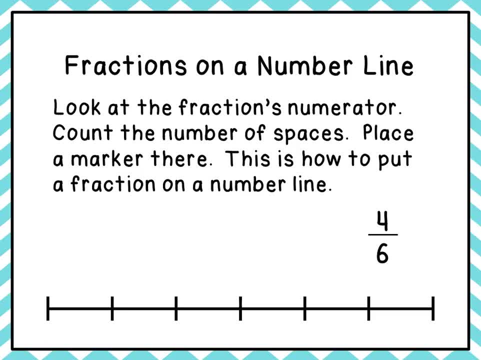 at the fraction's numerator and we're going to count the number of spaces and we're going to put a marker there to show that the fraction is. that's where the fraction goes on the number line. Our numerator here is four, So we're going to 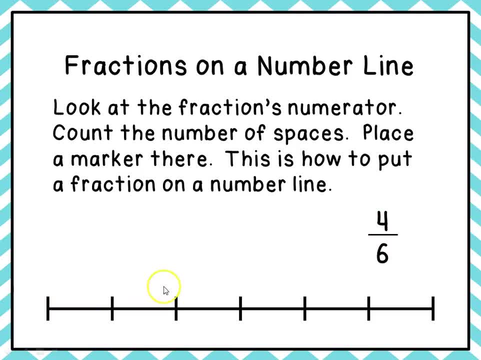 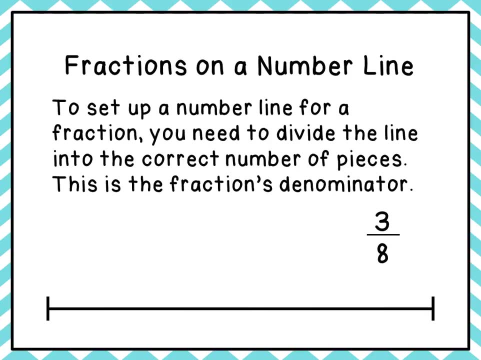 count four spaces. Here's one, two, three, four, And I'm going to put a marker right there to indicate that on this particular number line we're looking at four-sixth. There are six pieces and we counted four, just like in the numerator. Okay, Again to set. 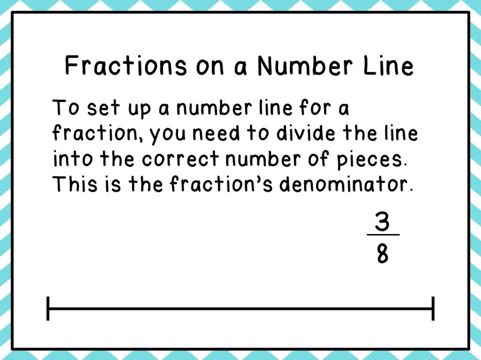 up the number line. we need to divide it into the correct number of pieces. that's indicated by the fractions denominator. In this particular one, we're going to divide it into eight different sections. So now we have two sections, three sections, four sections five, six, seven and eight. If you look here we got one. 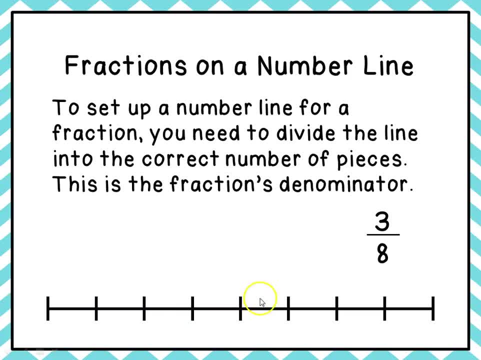 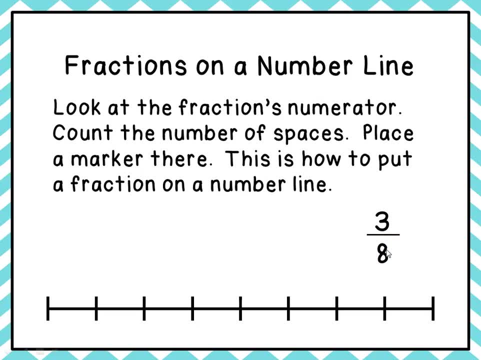 two, three, four, five, six, seven, eight, Just like you see there in our denominator. And then we're going to look at the numerator and we're going to count the number of spaces. remember not the lines. we're going to count the. 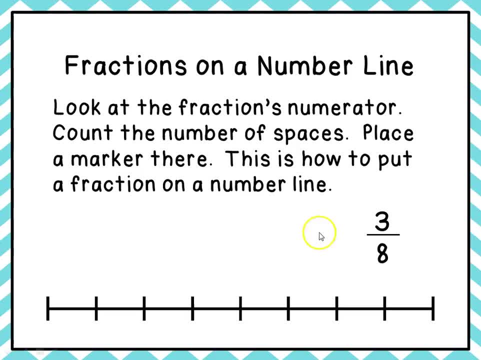 spaces that's shown in our numerator. In this particular case, since we're looking at three eighths, we're going to count three spaces- one, two, three- and we're going to put a marker right there to show three eighths. 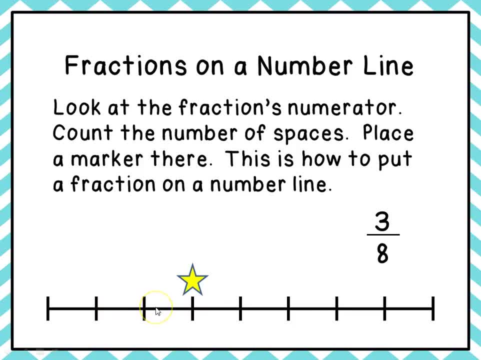 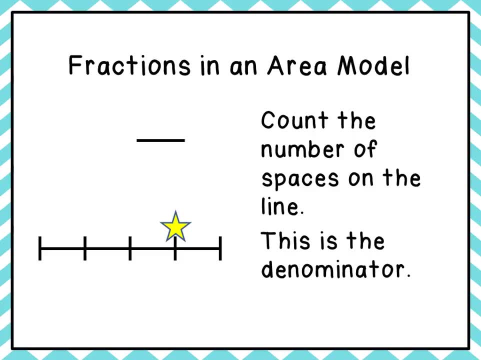 Eight spaces on the line all together, we marked off three of them. Alright, so let's do. what we want to do here is we want to figure out how many or what fraction we're looking at on this particular number line. So the first: 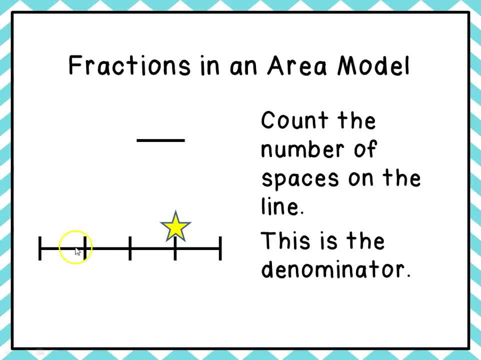 thing we're going to do is count the number of spaces on the line. So here's one, two, three, four. So our denominator is going to be four, And then we're going to count the spaces until we reach the marker: one, two, three. That is the numerator. so we put that there and 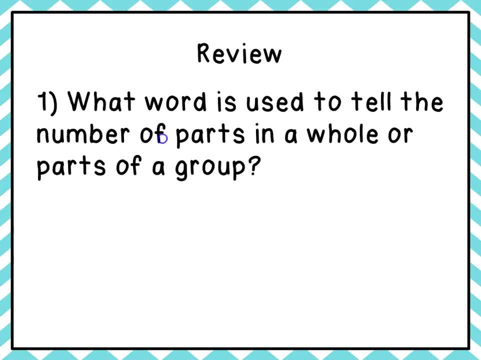 our fraction ends up being 3, 4.. Alright, so let's do a little bit of review here. Question number one: what word is used to tell the number of parts in a whole or parts in a group? Give you a second to. 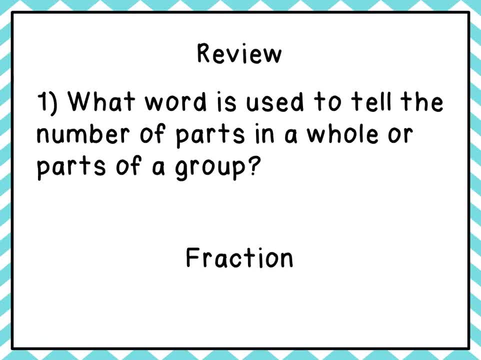 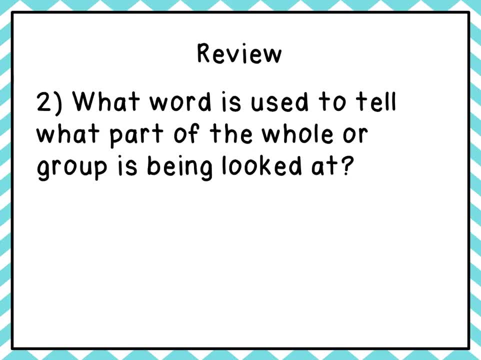 figure that out. If you chose fraction, you are correct. Question two: what word is used to tell what part of the whole or group is being looked at? and the answer here is the numerator. it's the number on top. tells you how many you're looking at. 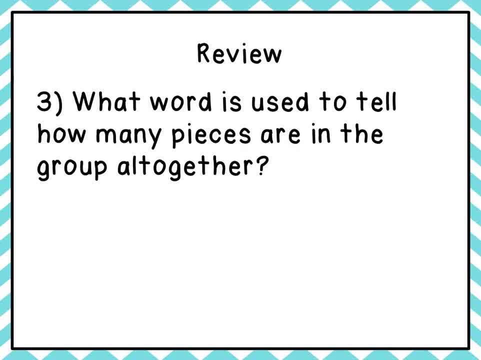 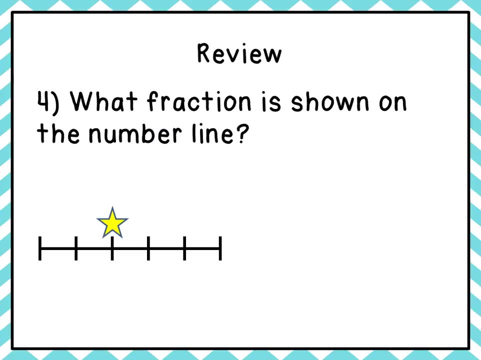 question three: what word, what vocabulary word, is used to tell how many pieces are in the group all together? that would be denominator. that's the number that we find on the bottom of the fraction. it's how many pieces we have in all. alright, let's take a look at this. question number four: what fraction are we going? 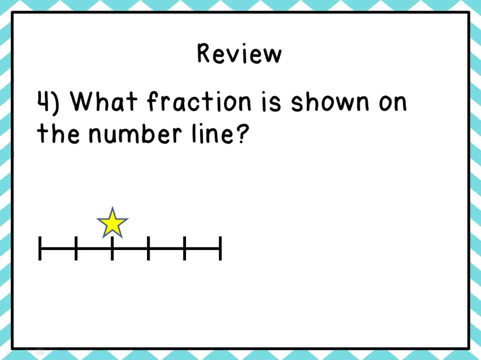 to see on the number line. well, the first thing we have to do, if you remember, is we're gonna count the number of pieces we have. so one, two, three, four, five, there are five pieces all together on the number line. that's our denominator, and then we're gonna count till we get to the marker one, two. so two is our. 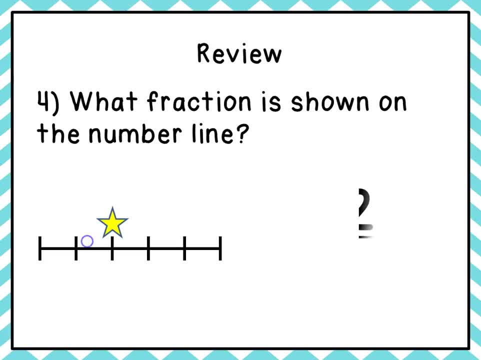 numerator. So the fraction you should be saying is two-fifths. Okay, question five. Here we go again. What fraction is shown on this number line? I'll let you figure this one out. Okay again, don't forget to count all of the pieces on the line.